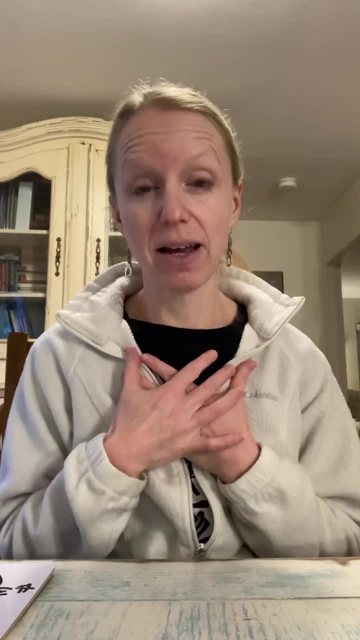 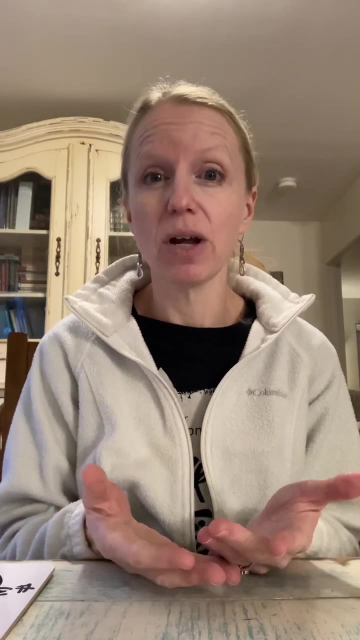 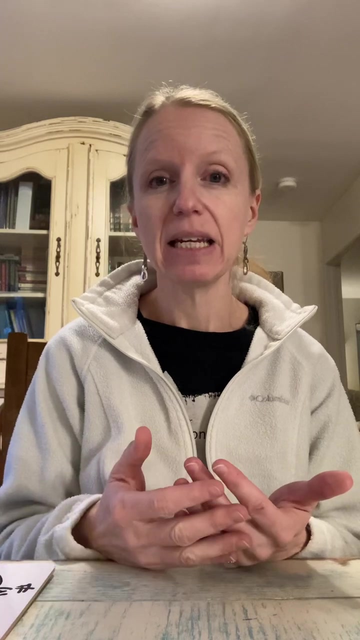 we cannot- well, i cannot at least yet make dialectical or rhetorical type conclusions, because we're just not there yet in our knowledge base. so just have fun with these experiments and just remember we're in the grammar stage of learning, so we're just learning the vocabulary. 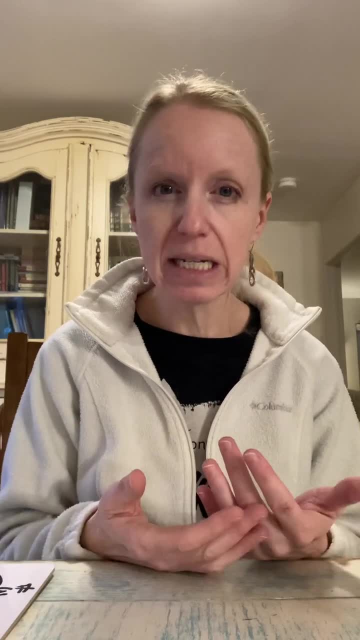 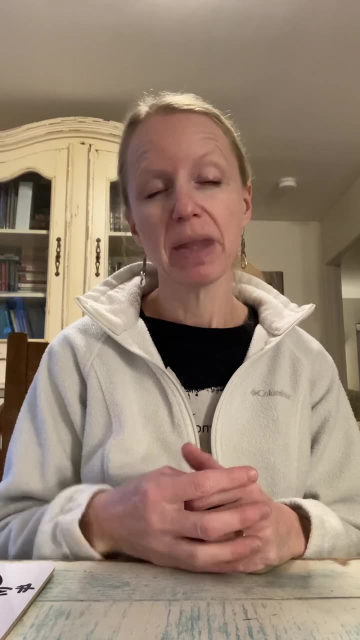 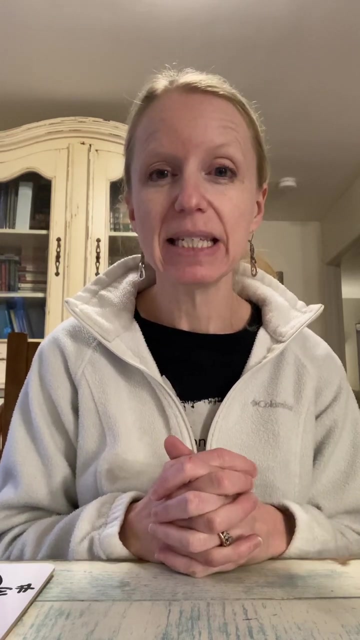 probability, distribution sampling. we're just learning definitions, we're practicing these things and some basic experiments and just having fun with it. we can build on that knowledge base later. so for distribution, um, this week we are doing the blueberry pancake experiment. our materials are very simple. 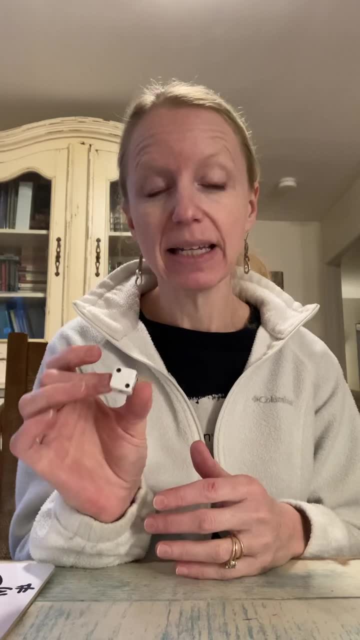 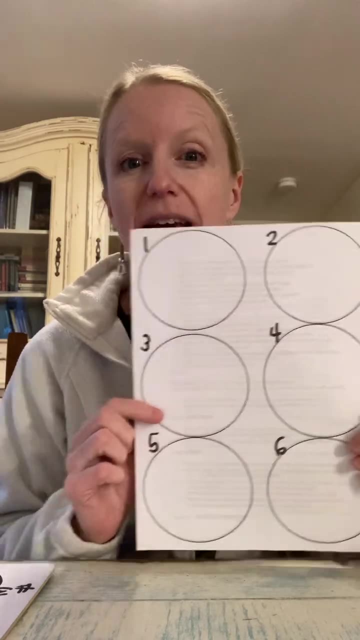 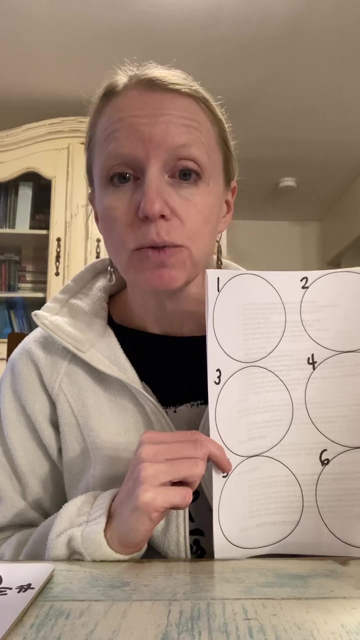 we'll have, um i'll have a dice enough for um the kids to work in pairs, and then you also have a blueberry pancake sheet for each of those pairs. um the experiments you're going to do, first of all as a class and a tutor um doing it up on the board, and then you're going to be able. 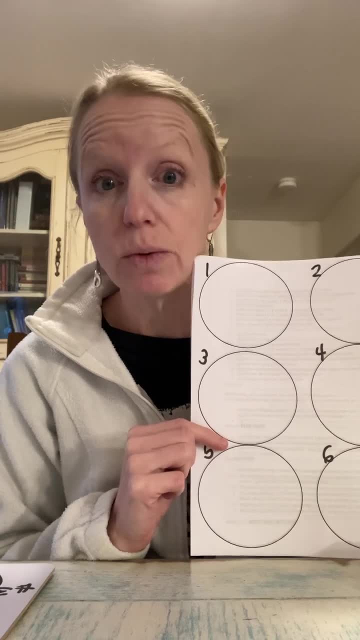 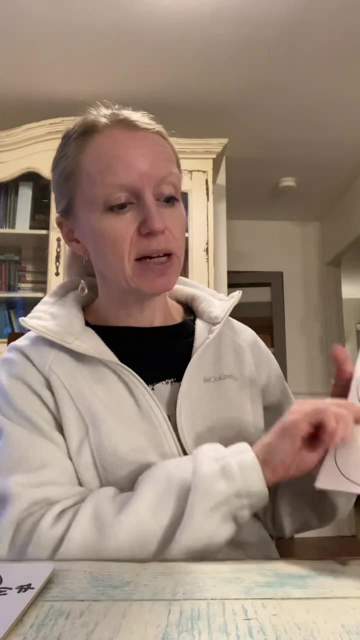 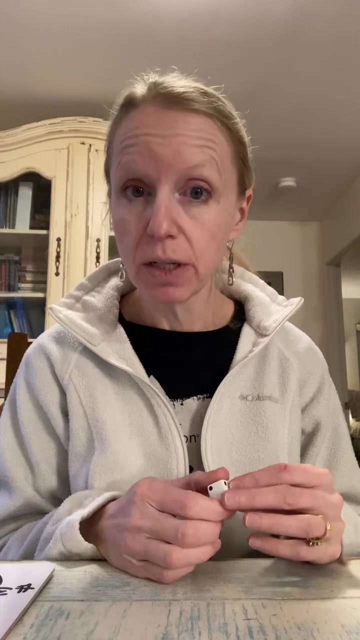 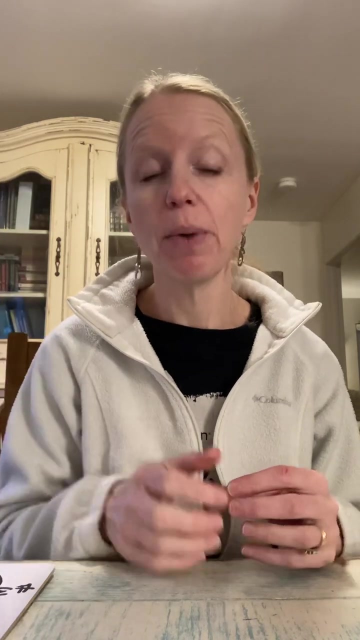 to break off in pairs or in the littles you can do: tables and have a parent per table, whatever works best. um, again, the idea with breaking off in groups is to get more results to compare your probabilities because we know to find your probability outcome. we look at our desired outcome over our total possible. 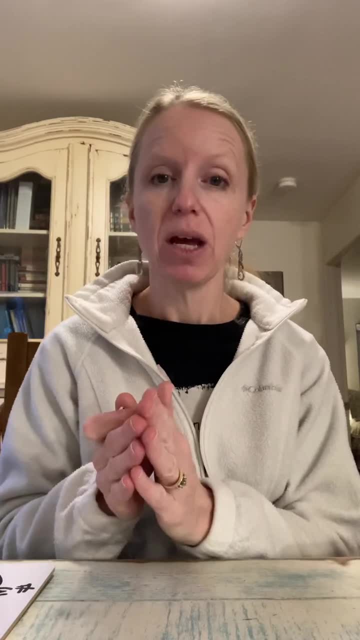 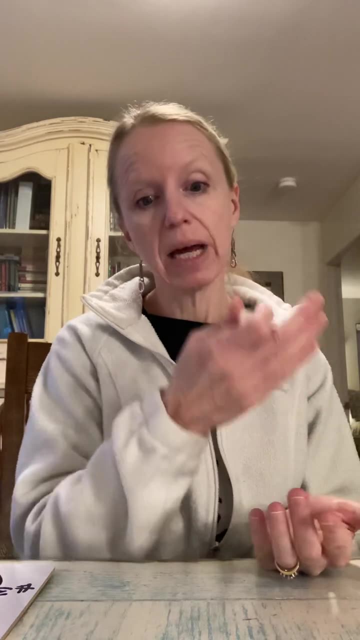 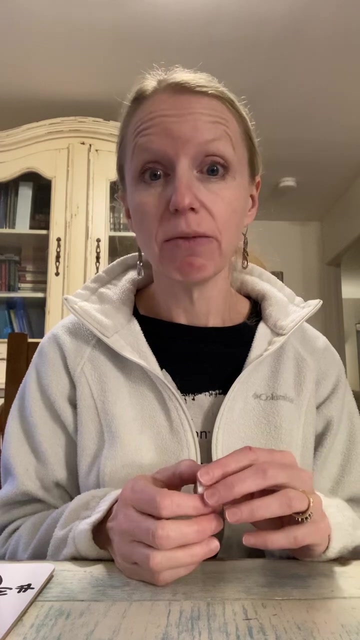 outcomes and our probability. our results of an experiment are not always equal to a probability, but the more attempts you do, the more results you have, the closer they are to an accurate probability of whatever it is you're investigating, and so that's the idea of doing it once as a 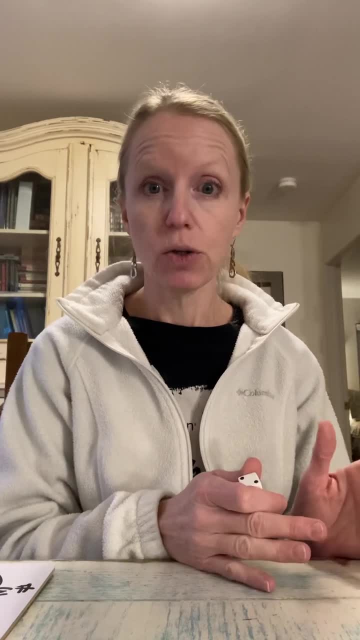 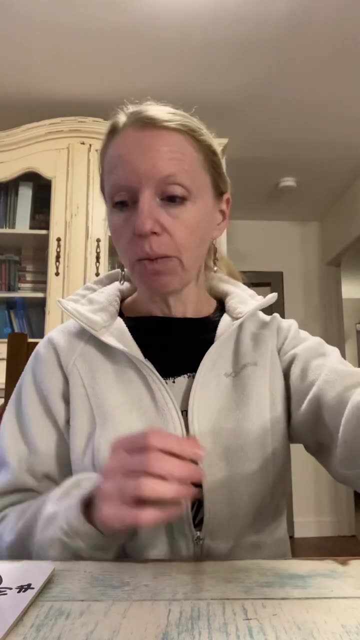 class to get an idea of what we're doing, and then breaking off into our pairs or groups to get more results, to get a more accurate probability. all right, so what we do, i've started the tutor demonstration ones. you don't have to watch me roll the dice 15 times, um, but you're just going to be as. fast as you can. so you're going to be as fast as ways if you just relax and study seriously. but- and this is going to help the trenoufledness exercise, so i'm going to push up a little bit more and then i'll change the score over it. so a little bit, yeah. so this daily would, before students, check out more videos. 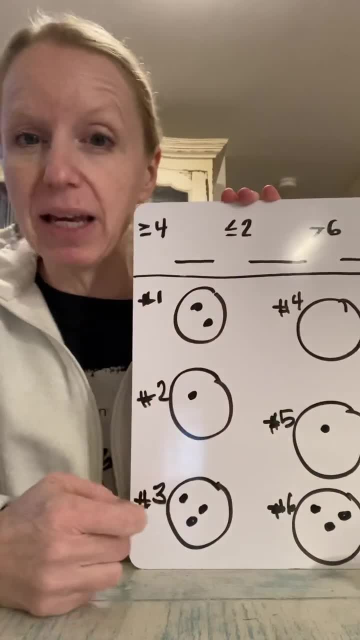 um, but my model is a this video like: if they want to do them all in rooms and then we can link to it then. But you're going to have first of all your six pancakes up on the board. You're going to number them one through six. 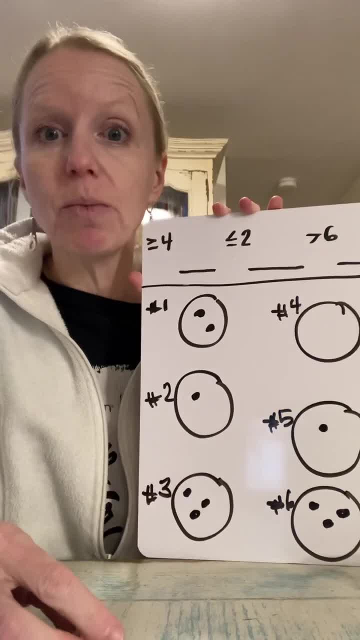 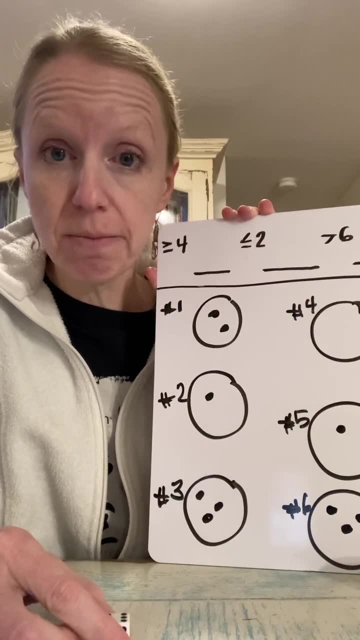 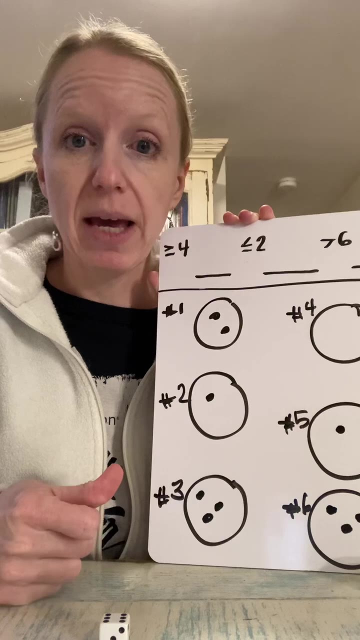 You're going to have your dice And the story goes that we are making blueberry pancakes. In our particular bowl we only had 15 blueberries, So we want to know what's the likelihood we will have at least four blueberries in our pancake. 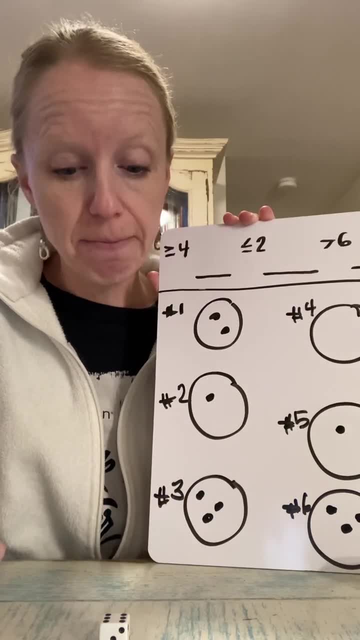 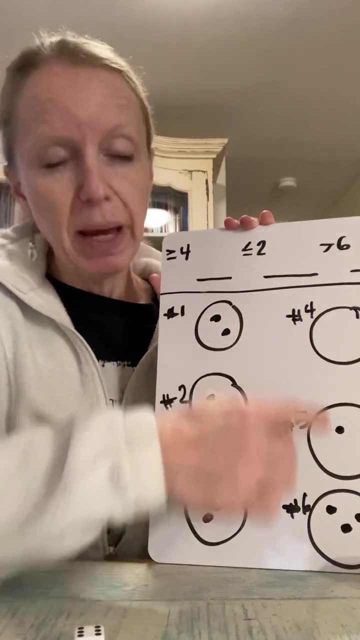 Because if you're making blueberry pancakes, they've got to have something in there, right? Okay, so when we roll the dice, depending on the number you get, it's the number of pancake that gets a blueberry. So I've already done 10 rolls. 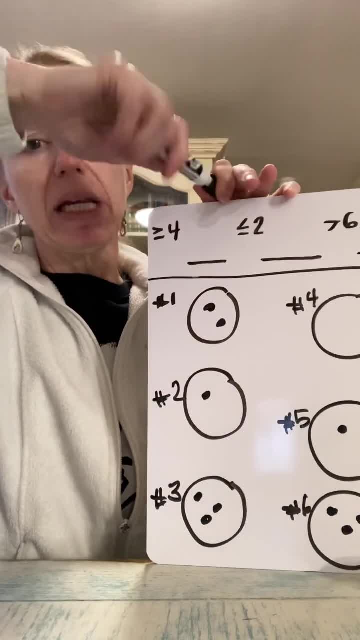 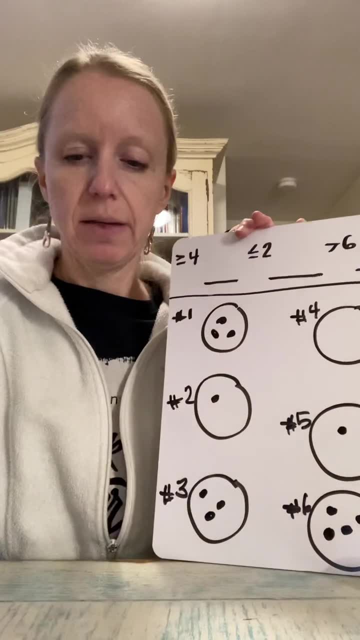 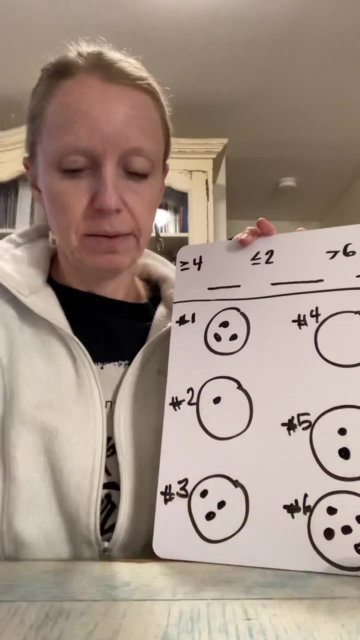 I'm going to do another one. I got a number six, So my number six pancake here gets another blueberry And a one, And, oh gracious, six, Five And four. Oh good, finally got one, All right. 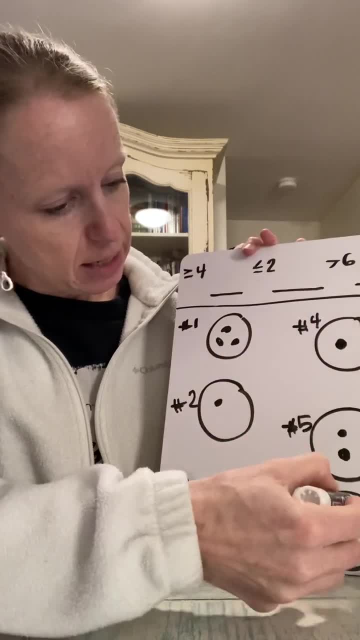 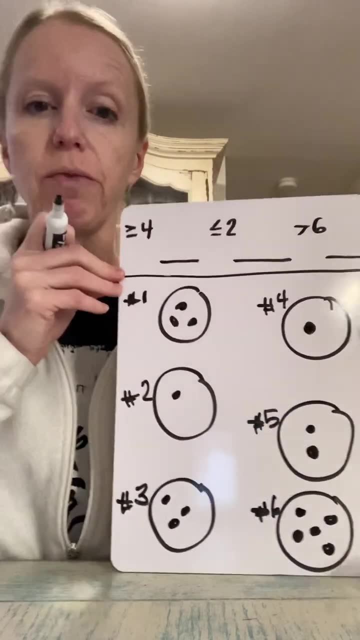 How many is that? Three, four, five, six, seven, eight, nine, 10,, 11,, 12,, 13,, 14,, 15.. All right, so I have my 15 blueberries now. So again, we've rolled it 15 times. 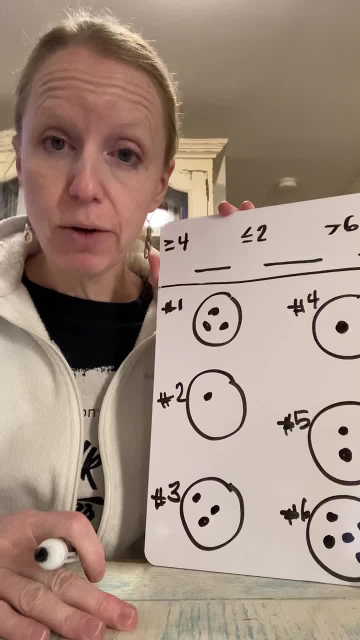 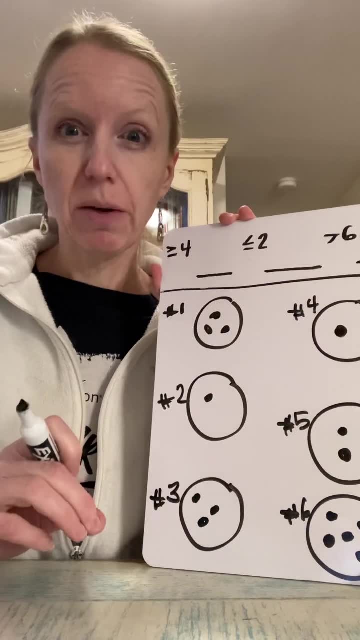 We've distributed our blueberries. Now we're going to look for patterns or the distribution of our results or blueberries. Now this is kind of a trick. I want you just to think about it As you're, as you're answering these questions. the question is: 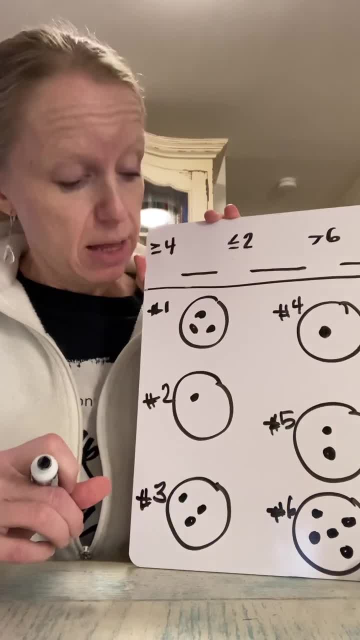 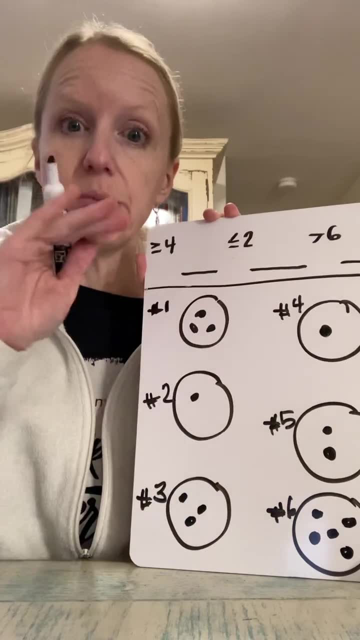 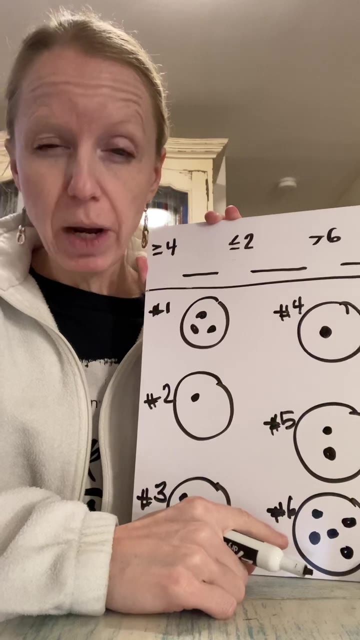 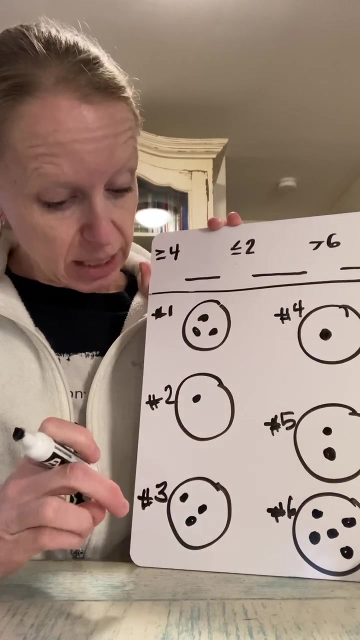 what is the probability or likelihood that our pancake will have more than four blueberries? So our desired outcome is more than four over our total possible outcomes, which is six, Because the question is about the pancakes. The question is not: how many times did I roll? 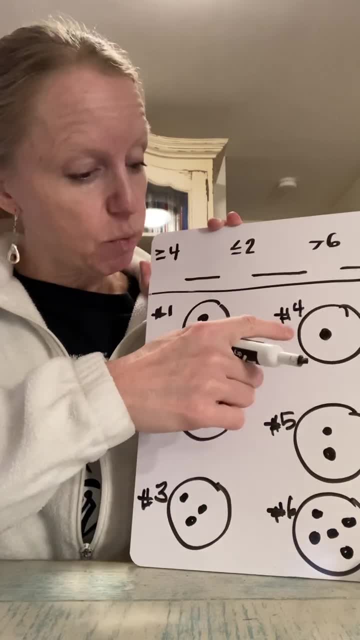 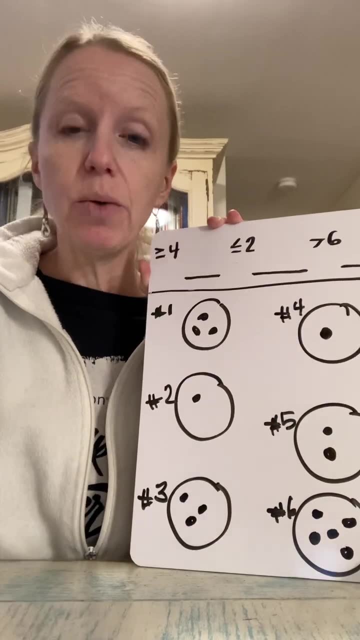 A number four, Or how many times did I roll a four, five or six? It's not about the dice roll like we did the first week. This is adding a whole nother factor into it with looking at a distribution or pattern. 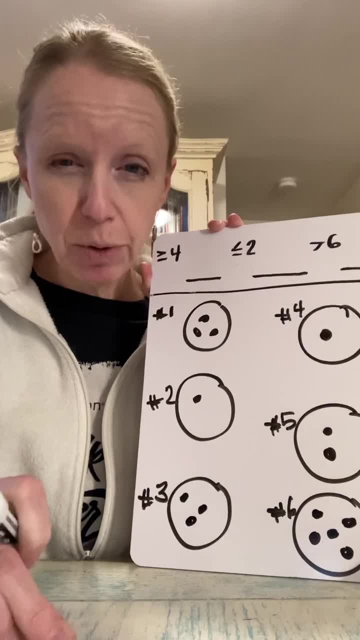 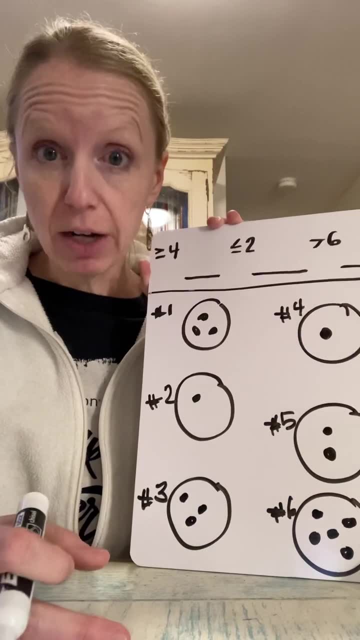 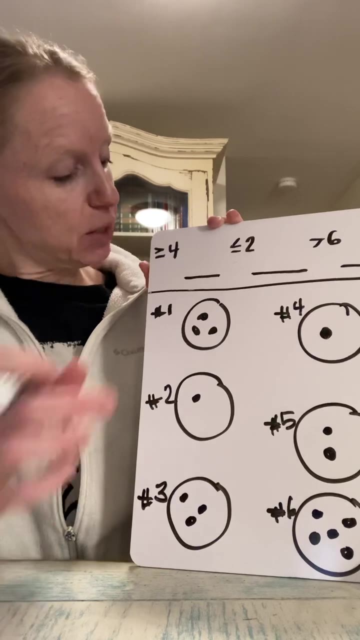 So, with the question we ask, the experiment we're performing will depend, will determine your, your probability fraction or how you pronounce or declare your outcome. So if we answer this question, how many pancakes? what's the probability of this first experiment? 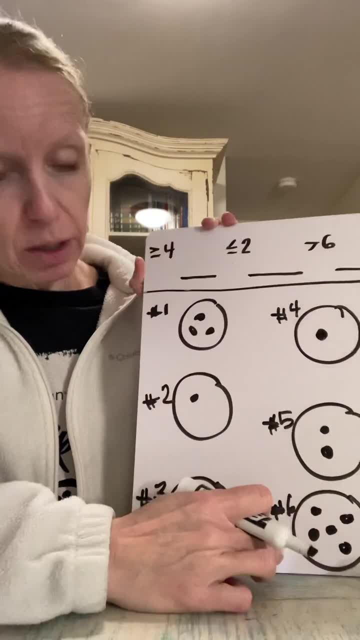 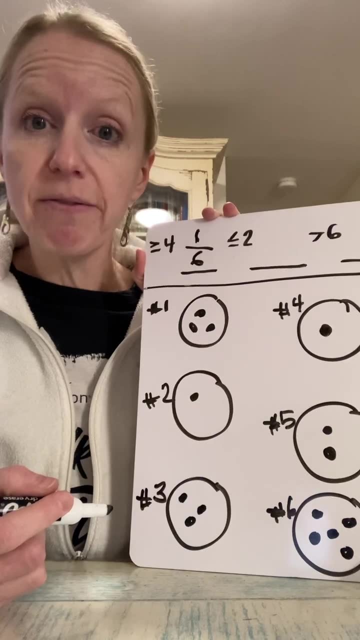 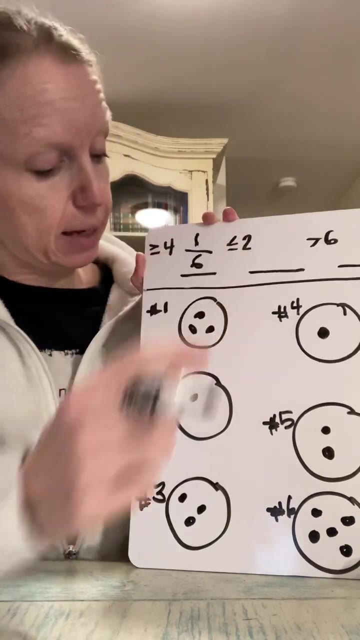 Will a pancake have more than four? Well, only one of my pancakes does So. one out of my six possible pancakes has more than four. How many have less than or equal to two? So have at least two pancakes or two blueberries. 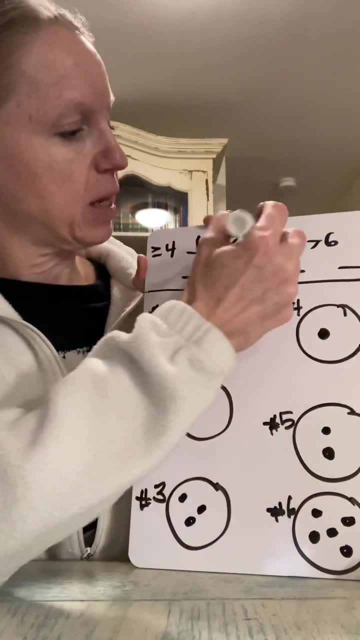 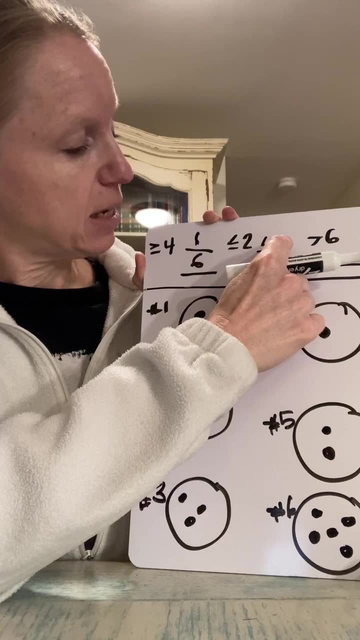 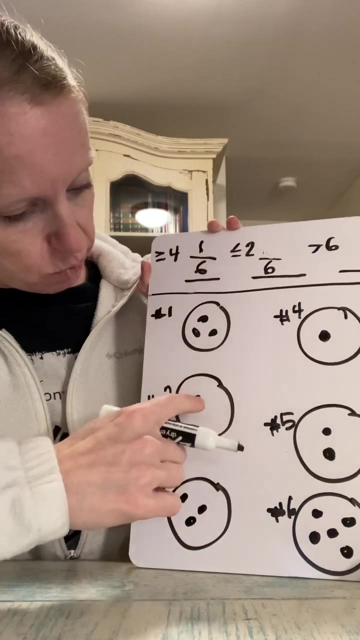 Sorry. One, two, three, four, So four out of six. So again my desired outcome. So less than or- oh sorry, Did that wrong- Less than or equal to two would be one, two, three, So three out of six. 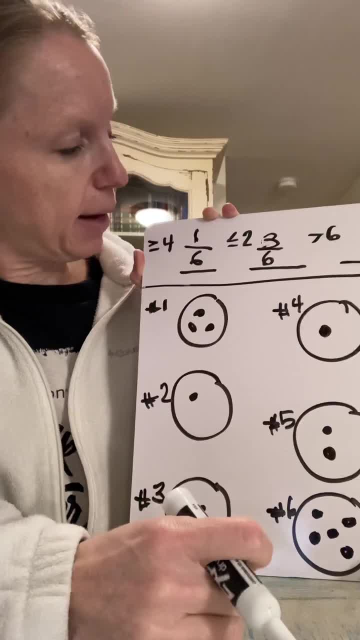 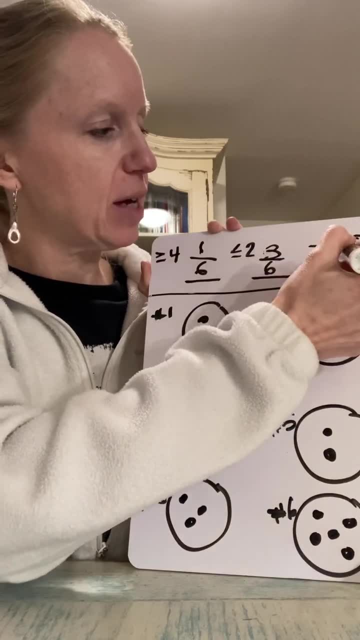 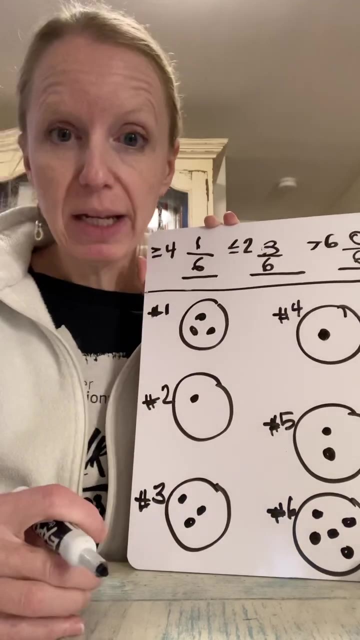 So three out of six have less than or equal to two pancakes or two blueberries. And then how many have greater than six Zero. My desired outcome over my total Possible outcomes are six pancakes, And so those are some probabilities or outcomes that we can determine from this particular thing. 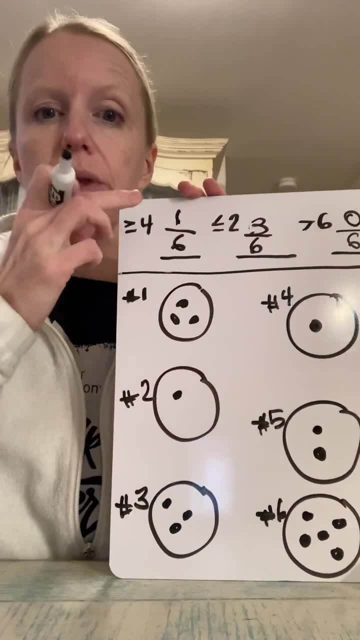 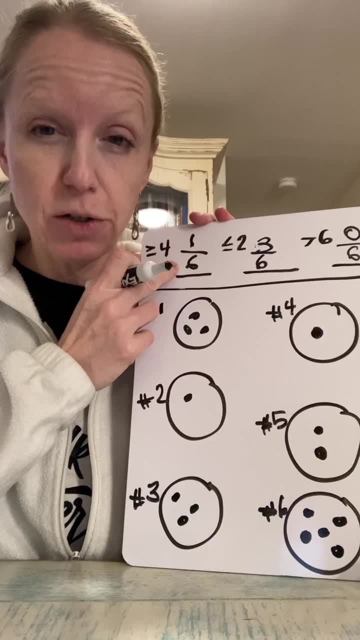 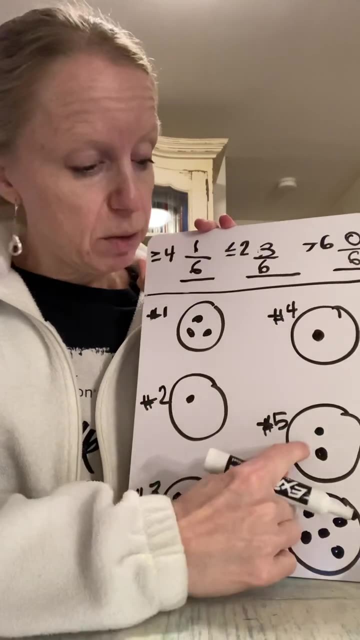 So, so again, the, the answer for, especially for your denominator here, is going to be the number of pancakes, Because that's the question we're asking. Versus, if I said how many times did I roll the number five, It would be. 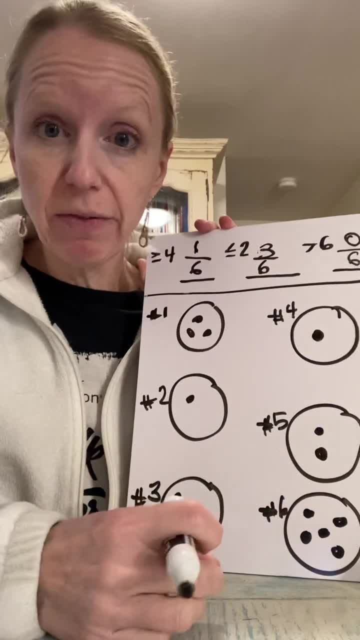 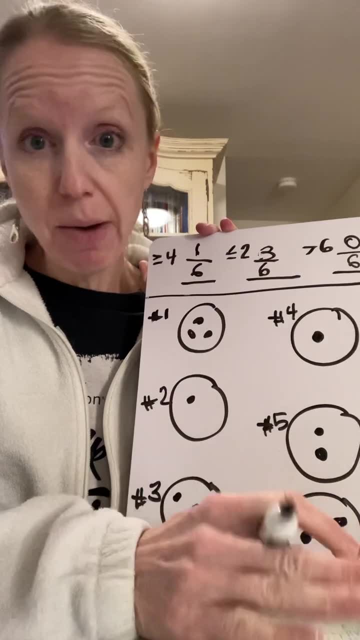 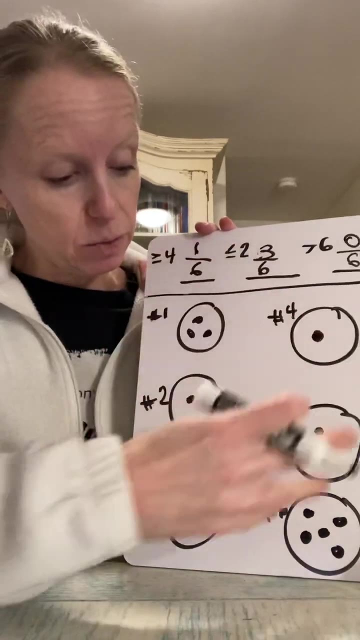 Two out of 15, the total times I did it would be 15.. The number that my desired outcome of number five would be two out of 15.. But that is not my question. My question is: which pancake? how many times did a pancake get this? 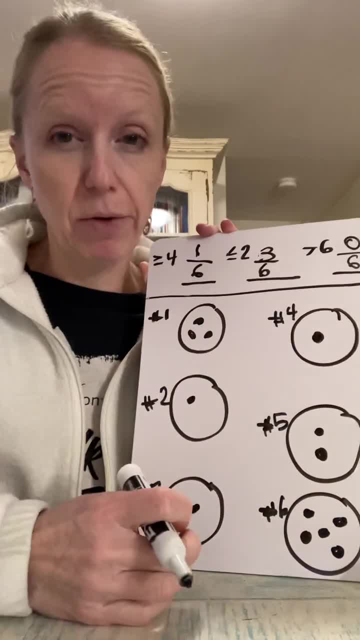 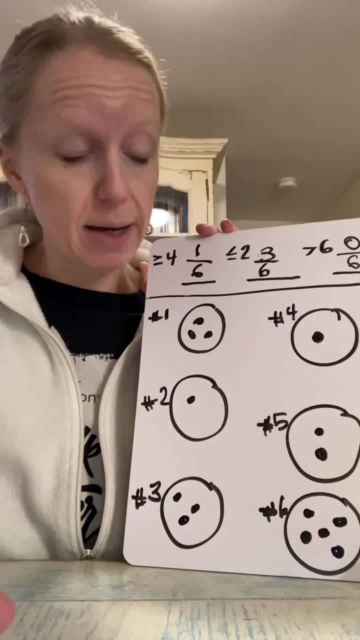 Well, out of six pancakes, my desired outcome is whatever. So I hope that makes sense. So we're. we're taking it a step further than where we did the first week, when we were rolling the dice. Um, okay, So this is the Tudor ones. 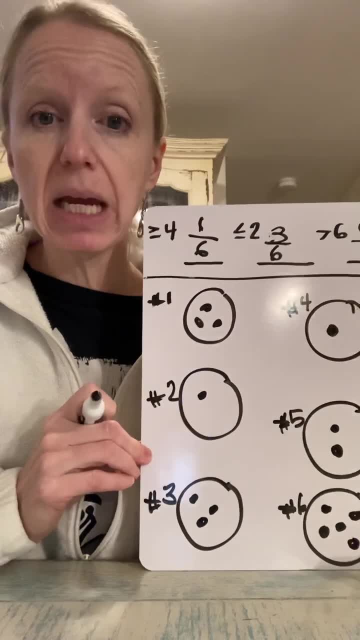 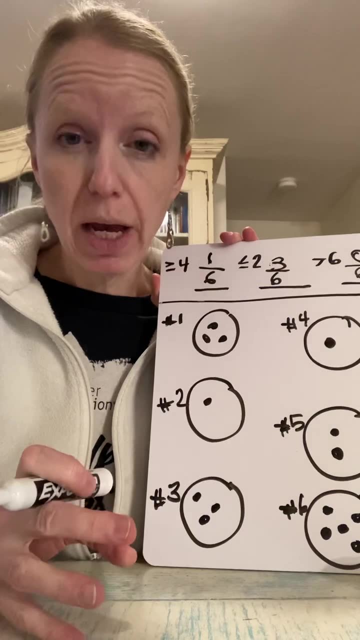 You're going to just show them basically, um, the idea. here And again we're looking for patterns, So um, and this idea of distribution. there's also this idea of outliers, So things that don't fit the pattern. 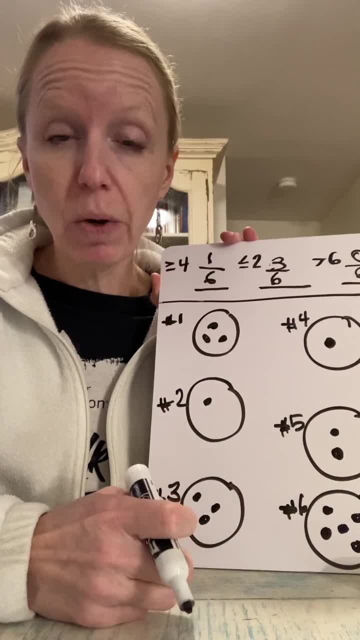 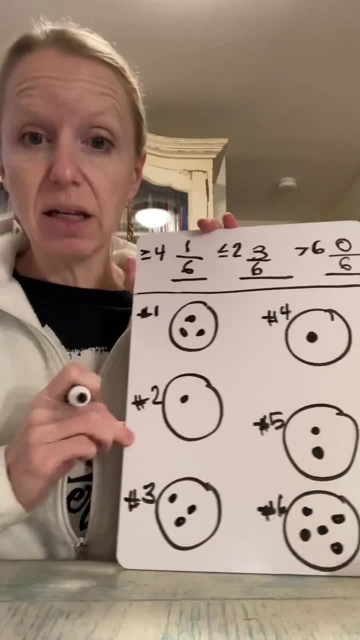 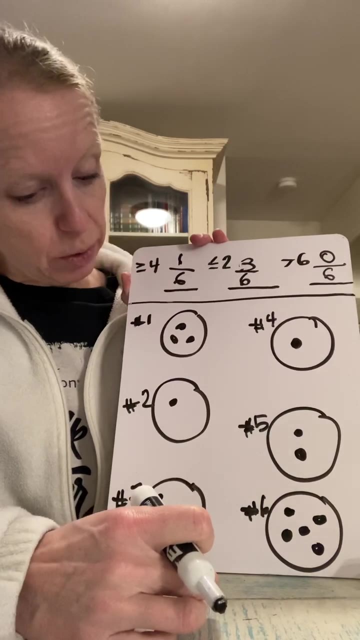 So you could look at just my one, you know one time of doing it and say: is there anything that looks like an outlier to you? Um well, number six has a lot more than the rest, So the likelihood of getting you know five or more is still one out of six. 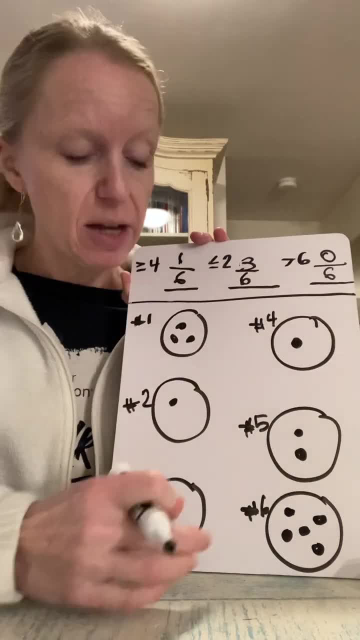 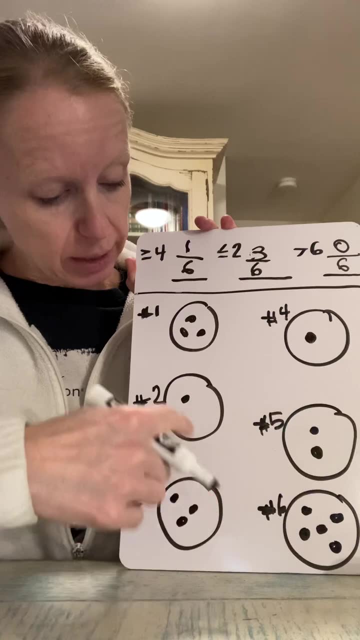 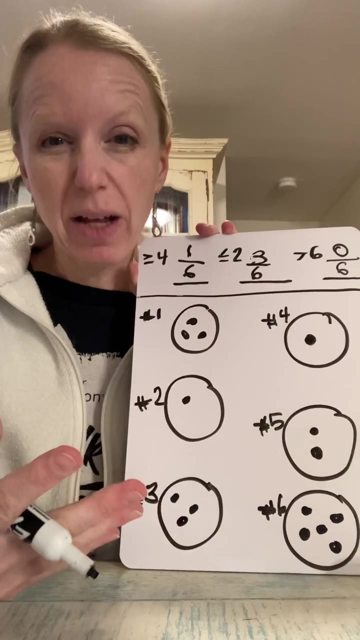 Um, so I guess you can really say that that is, but as each kid is doing them, as you're getting a group, if one group got, you know, all got 10 and the second pancake and zero and some of the others, that would be an outlier. 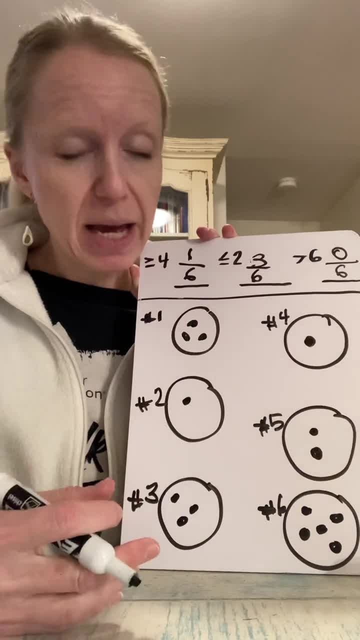 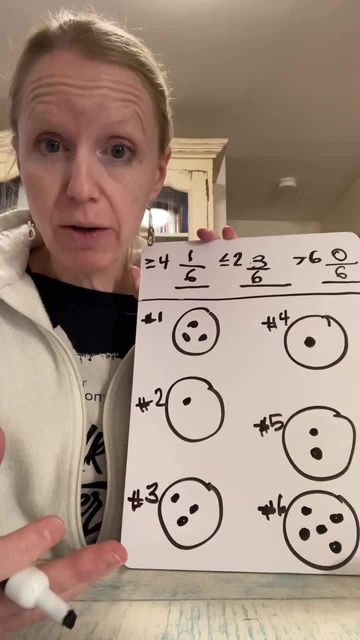 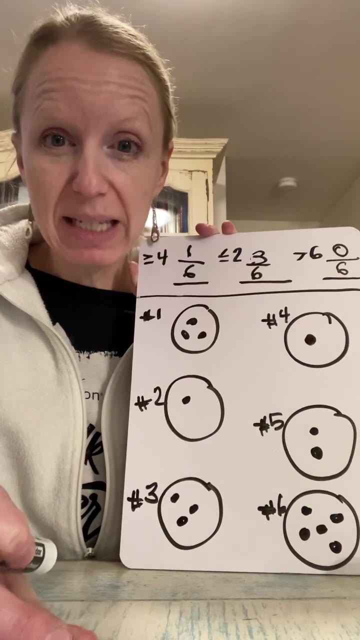 So their results can still be counted. but they may skew your Um and so because their distribution or their pattern was not similar to everybody else's Um, so sometimes those outliers will happen: Um, our dice can, um can do that. 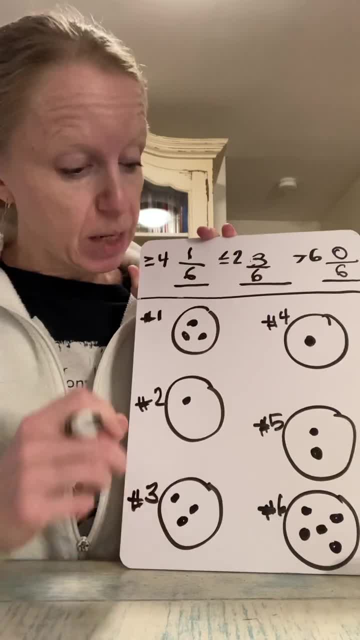 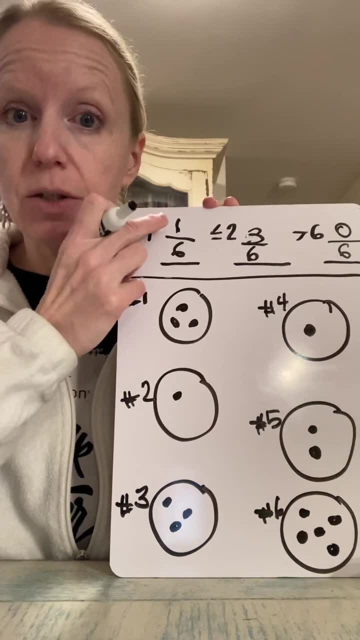 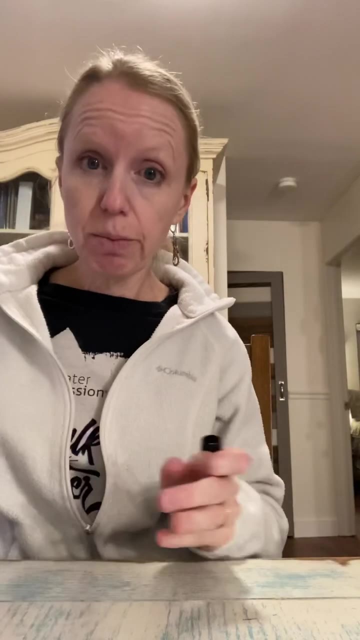 And that does skew or throw off our our results. So, Tudors, are going to do this again And make sure you clarify: our probability is total desired over our possible outcomes, which are out of our six possible. And then each pair or table will have their set of six pancakes and their dice. 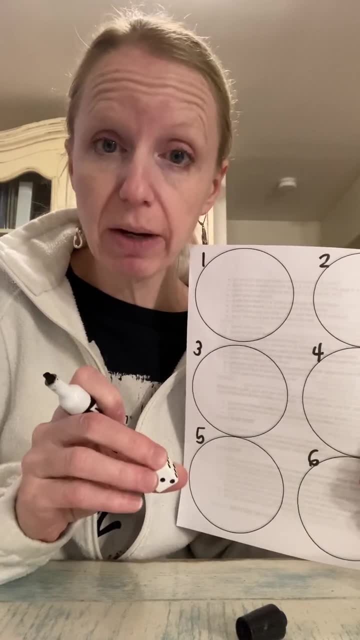 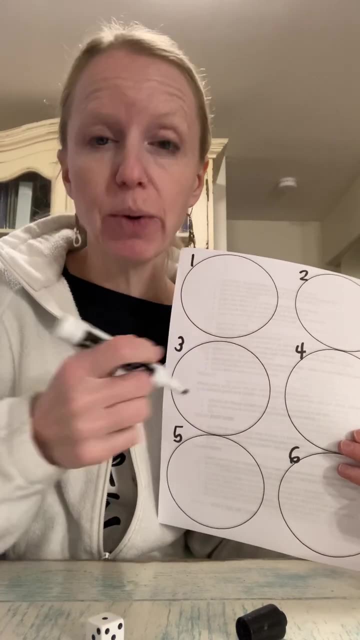 They're going to do the same thing. You're going to have 15 possible blueberries that will be distributed amongst your pancakes, Um, they can put. use their pencils to put a dot, just like you did on the board, Um, and then, together as a class, you're going to do the same questions. 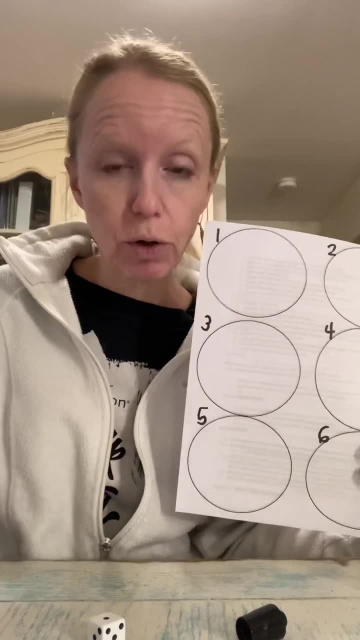 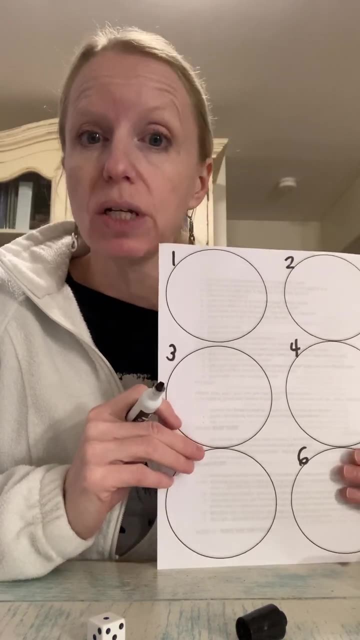 So, um, how many you know? go group to group, How many, How many of your pancakes had more than four? And then write your results up on the board and see if you start to see a similar pattern. um, with more results.